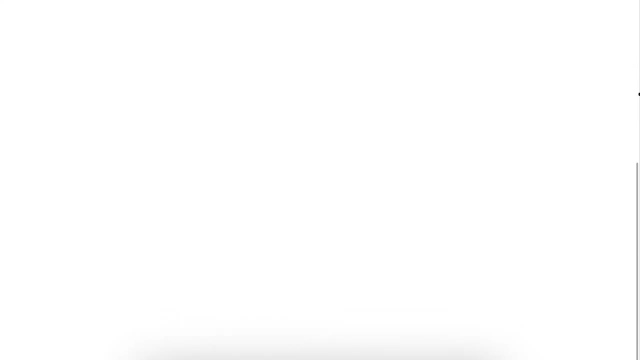 exercise. In the first problem. we consider the following scenario: Let's say that you just bought some chickens- One, two, three, whatever number- And you want to give them a specific part of your garden to roam around in. Therefore, you need to make some fencing, And you remember that in your shed. 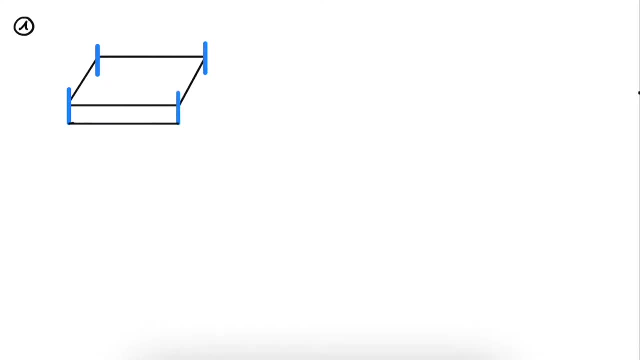 you still have some fencing left from some other gardening project. So you go and you look and you see that you still have 10 meters left of fencing and four poles. And with this fencing and these four poles, you decide to make a rectangular area in which these chickens can roam around freely. 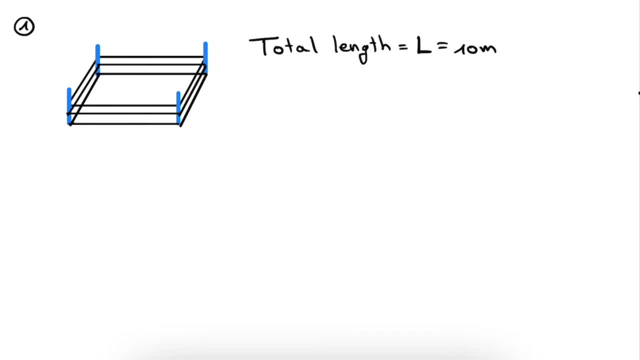 And with this fencing and these four poles, you decide to make a rectangular area in which these chickens can roam freely And with the well-being of your chickens in mind, you pose yourself the following question: Given that the total length of the fencing is 10 meters, what is the largest? 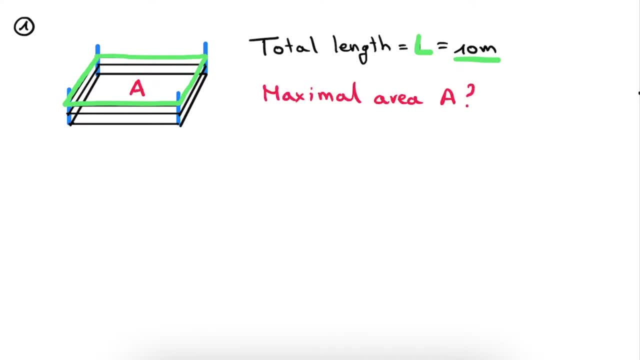 area within this fencing that you can make, given that it has to be a rectangular fencing? Or, in more abstract terms, what rectangle with a circumference of 10 meters has the largest surface? So let's put this down more precisely So we know that we are dealing with a rectangle. 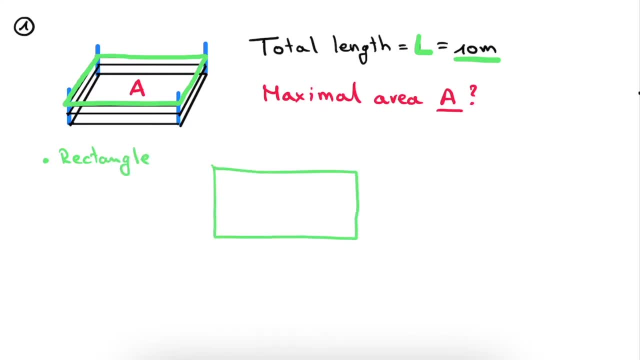 which is a fencing, And we know that we are dealing with a rectangle, which is a fencing that is well, of course, characterized by its four right angles and, moreover, by its length and its width, And, given its length and its width, you can determine the rectangle. So the question now is: 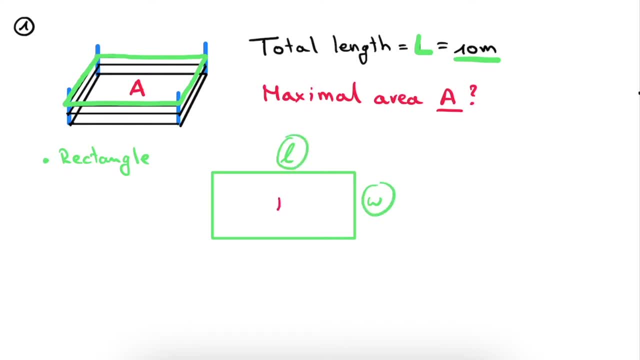 what length and width give the largest surface? A, given that the circumference of the rectangle is 10 meters. All right, So the first step is to identify that the area of a rectangle is, of course, the length multiplied with the width And, in the language of functions, which is the language that 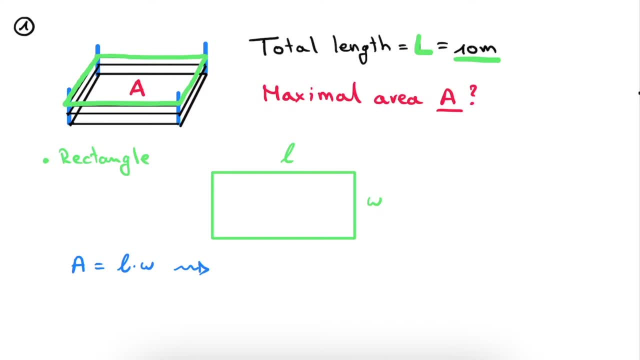 we need if we want to solve this problem using derivatives. this means that the area of the rectangle is a function of two variables: the length and the width. Namely, if we change the length, the area changes. Or if we change the width, the area changes as well. So what do we? 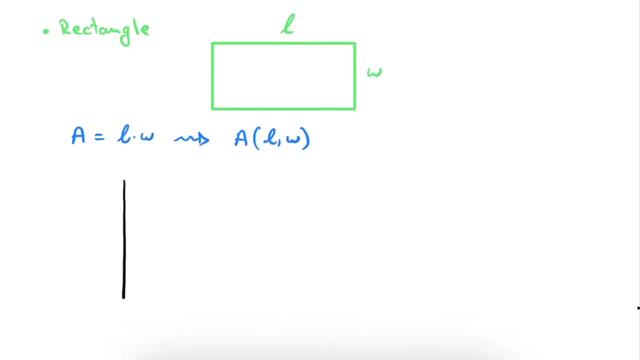 know about derivatives. Well, we know that graphically, the derivative of a simple function in one variable, for example x, represents the slope of that function. For example, if we take this point right here, the derivative of this function in this point will: 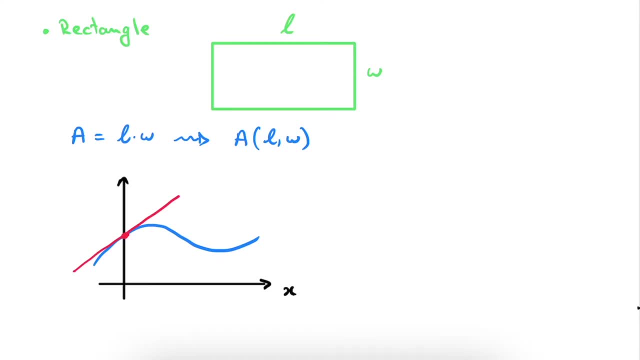 be positive because it has a positive slope. A natural consequence of this is that the maximum or minimum- but let's take maximum in this case because it's more applicable- the maximum of a function, for example here, will have a derivative that is zero, because in the maximum 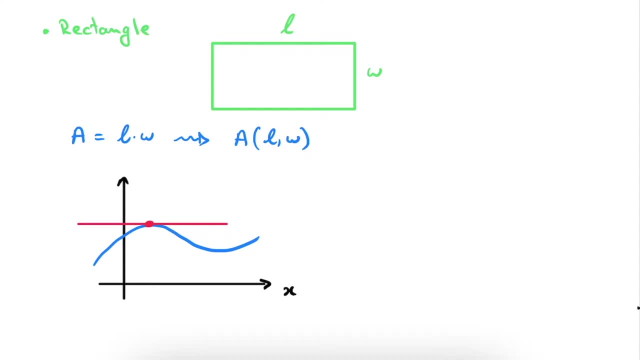 the slope of the function is zero. It goes from ascending to descending and therefore the derivative of this function in this point will be equal to zero, And that's how we identify the maximum of a function, And this, of course, very well suits our problem here. Why? Well, we want. 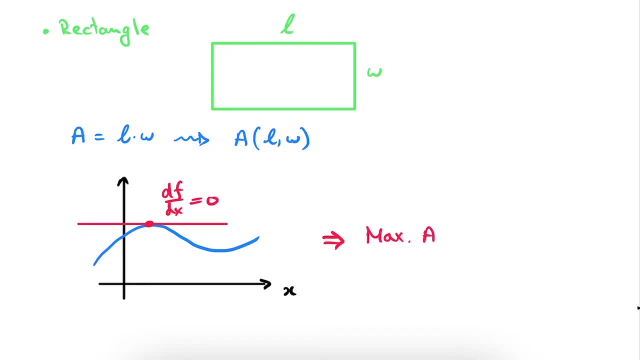 to find the maximum surface of our rectangle. And since the surface of our rectangle can be written as a function of two variables, we can find the maximum of a function of two variables. However, of course, this poses a problem because we have two variables: We have L and we have W. 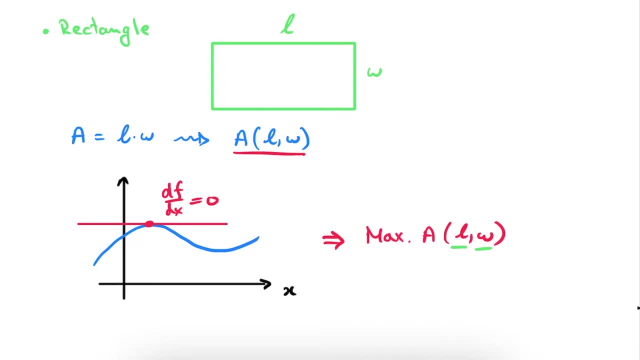 the length and the width. So does this mean that we have to choose whether to derive to L or to derive to W in order to find the maximum? Well, no, Making a choice between one or the other will not give you the right result. What will help you in this case is to transform this function of 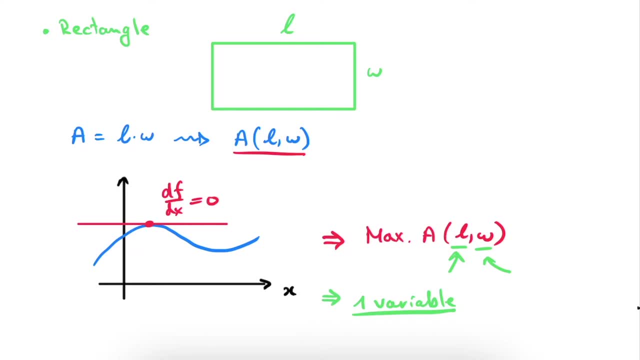 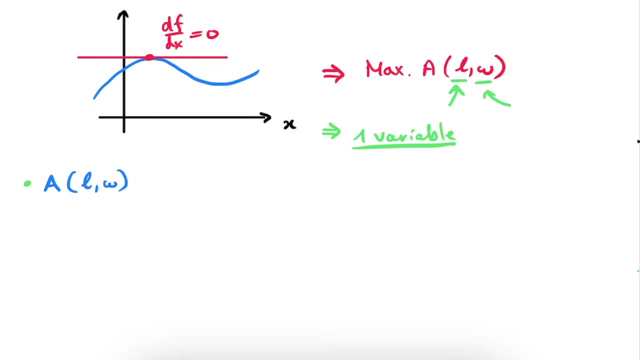 two variables into a function of two variables, And that's why we have to find the maximum of a function of one variable, And this is exactly what we will do next. In a nutshell, we want to go from A as a function of L and W to a function A of just one of them, So we want to eliminate. 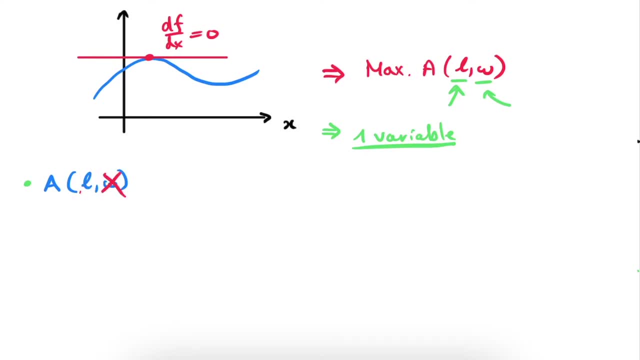 one of these two functions. Let's say that we want to eliminate W, It really doesn't matter. So what piece of information in our problem here didn't we use yet and will give us some more information about the problem, Or, in other words, will give us a constraint? Well, 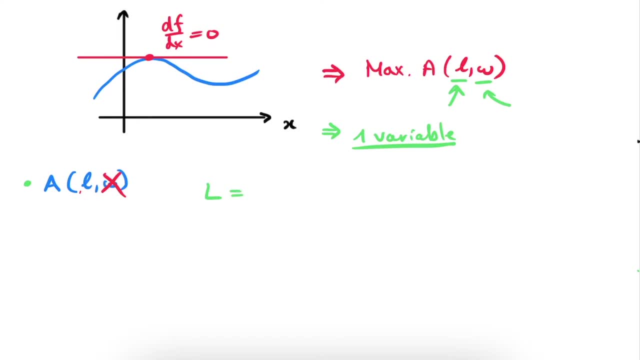 we did pose in the question that the total length of the fence or the circumference of the rectangle that we're trying to find is exactly 10 meters. And well, this is indeed a constraint, And we know that the length of a rectangle is equal to the length plus the length plus the width. 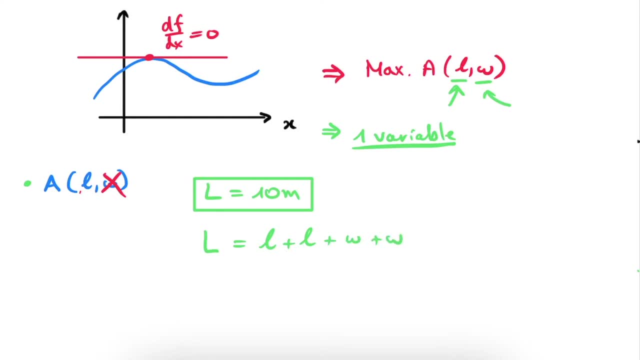 plus the width, So just the addition of the four sides of the rectangle, or, written differently, two times L plus two times W. And now we see that we have an equation which involves the two variables that we have and of which we want to eliminate one and one number. 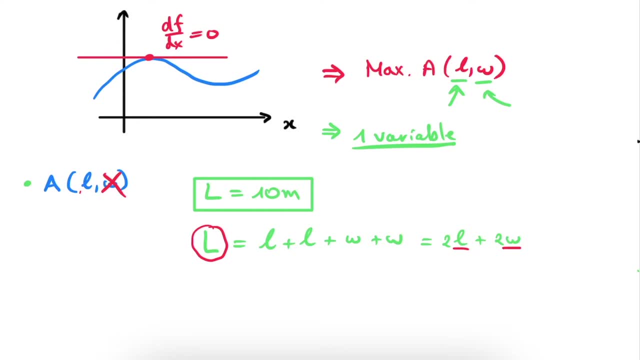 which is our constraint. In this case, the circumference is 10 meters, So we can rewrite this equation in the following way: W is equal to capital L divided by two minus small l, And in this way we indeed wrote W the width of the rectangle. 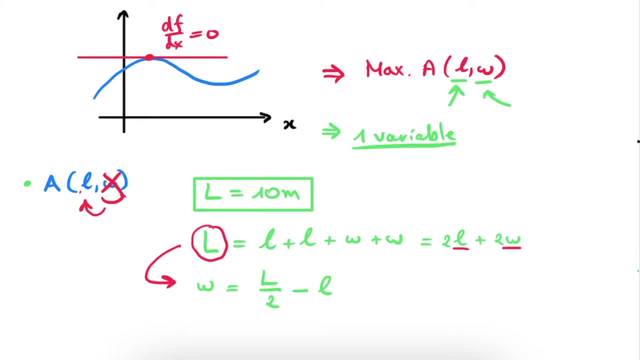 as a function of the length of the rectangle And of course, this capital, L, which is the circumference of the rectangle. But this is just a simple constant. So we've written one variable as a function of the other variable And this we can use now to rewrite our 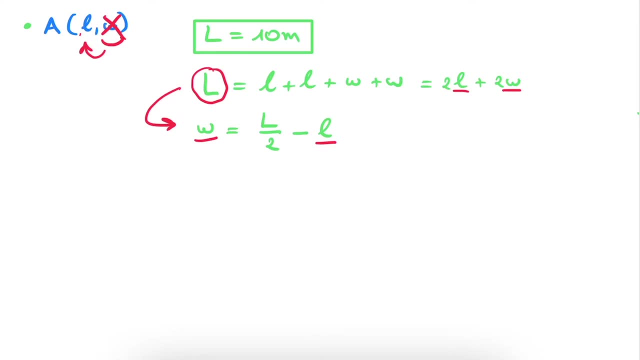 equation for the surface of our rectangle. And just to remind yourself, the surface of the rectangle is the function that we want to derive in order to find the maximum. Let's write our function of the area of the rectangle again, So we know that this is a function of two variables. 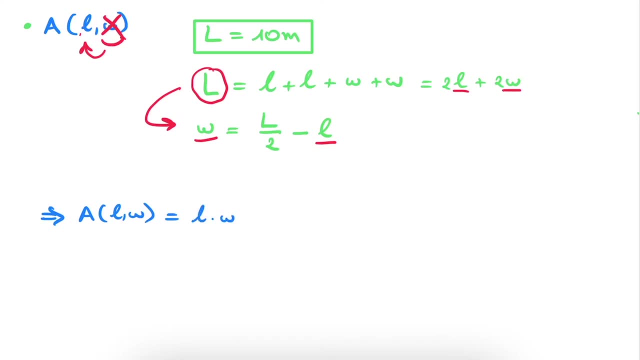 L and W, And it was simply equal to L multiplied by W, the length of the rectangle multiplied by the width of the rectangle. However, now we see that we can rewrite this width of the rectangle as a function of the length of the rectangle. 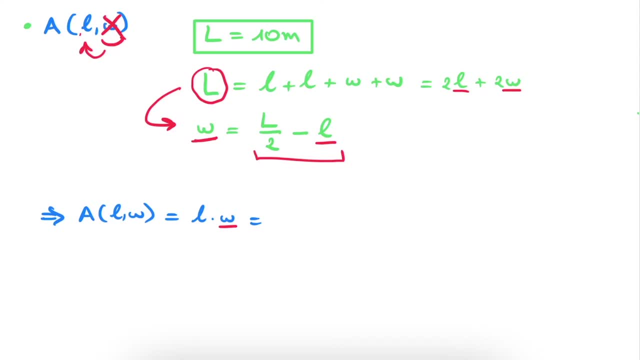 So we simply substitute this equation that we got from the constraint that we had. So we have small l, which we just copy, and then we multiply this with capital L divided by 2 minus small l, And we can, if we want, rewrite this even further as L multiplied by capital L divided. 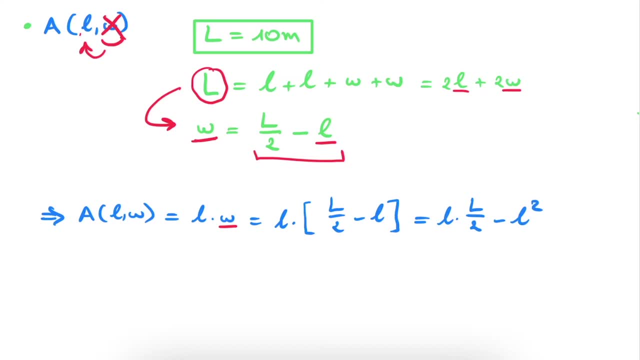 by 2 minus L squared, And we see that we've now written our surface of our rectangle as a function of one variable, namely simply L. And this is of course exactly what we wanted, because at this point we have a function of one variable, a, as a function of L, which we can now derive: 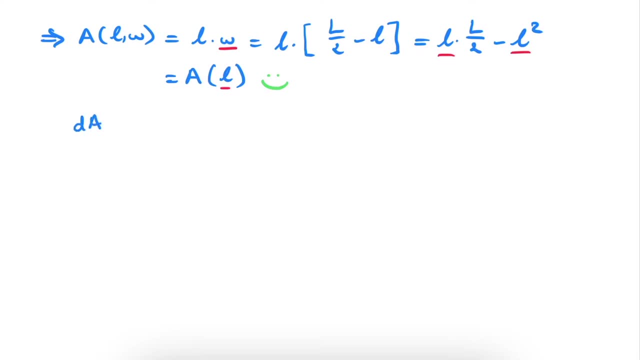 So we have to find the maximum, because we know that the maximum of this function, a of L, comes at the point where our derivative is 0, so where the graphical representation of our function has a 0 slope. So what we have to do is simply derive this function. 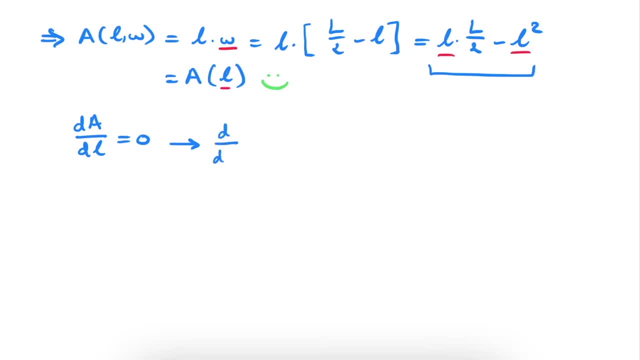 And we know how to derive it right. So we have to derive to our variable L the following function: capital L divided by 2, multiplied by our variable minus our variable 7.. And we do that by multiplying the variable by 2.. 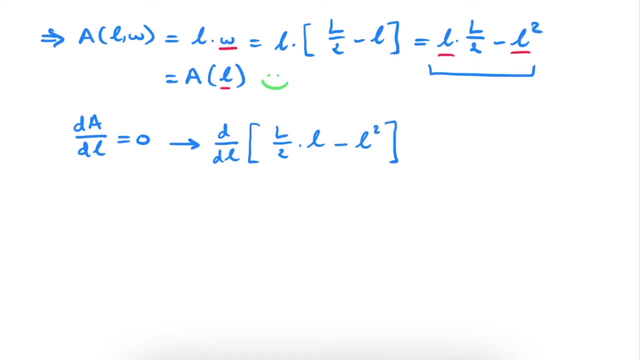 So this is our variable and we can now derive this function as well. We can now derive the function as well squared, and this is a very straightforward derivative, because this simply becomes l divided by 2, because this can be seen as a constant coefficient minus 2 times l, because 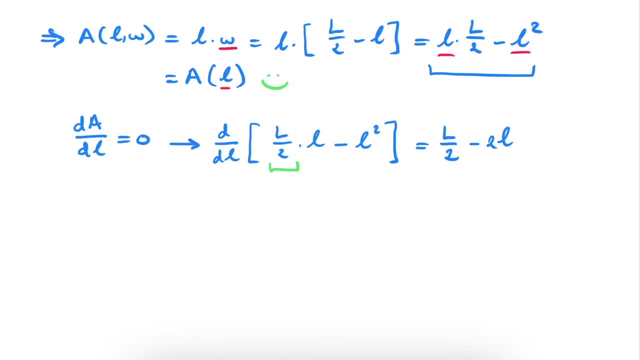 this square drops in front of it and the exponent drops by 1, and this expression will be 0 when our surface is at a maximum. so we simply have to solve this algebraic equation now, which is done as easily as the derivative we have. capital l divided by 2 is equal to 2 times the length of the. 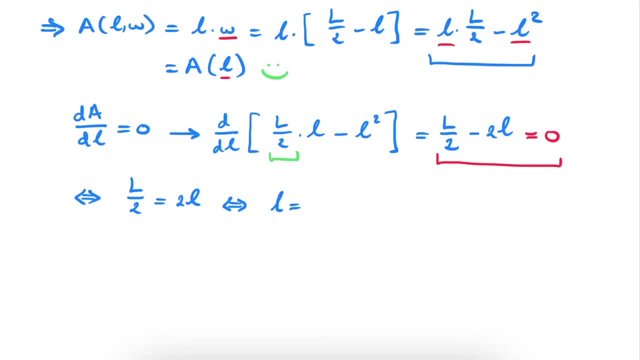 rectangle, or we have our final result that the length of our rectangle is equal to capital l divided by 4, and this is the result for the length of the rectangle, such that the area is at its maximum. now, remember that we earlier found a relationship between the width of the rectangle. 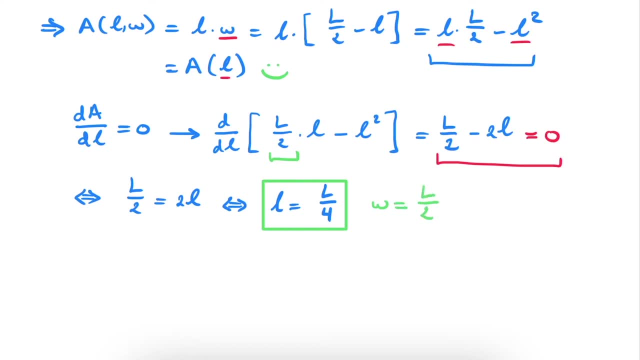 and the length of the rectangle, which was simply l divided by 2 minus the length of the rectangle, and we can use this now to find that the width of this same rectangle, which has a maximal surface, is equal to also l divided by 4, so at 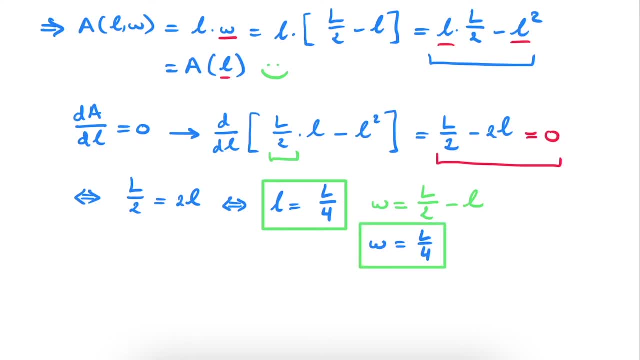 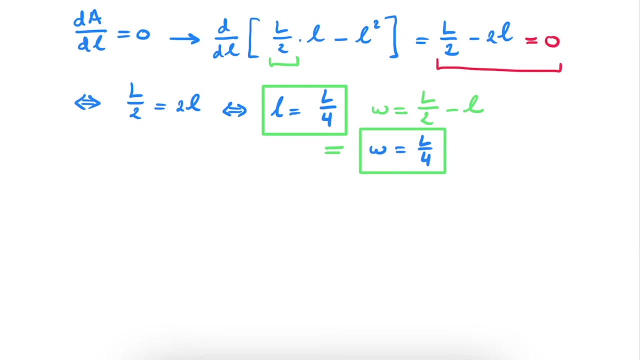 this point, we have the width and the length of our rectangle, such that the area is maximal. but do you notice anything? well, we see, first of all, that these two are actually equal to the length and the width of the rectangle we're actually looking for, are equal to each other. now, as you probably know, when the width 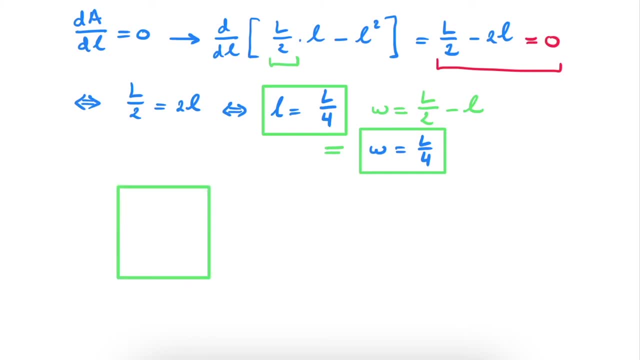 and the length of a rectangle are equal to each other. we simply have a square, and this is exactly the solution that we find here. we find that the length is 2.5 meters and the width is also 2.5 meters, and of course it checks out, because if we add all of the sides of the square together, 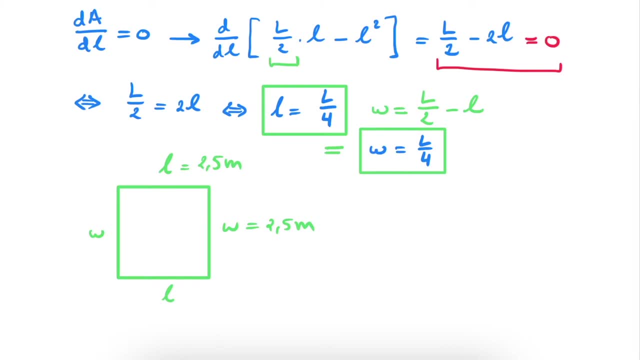 and, by the way, a square is also a rectangle- then we find, indeed, that the total circumference is 10 meters, exactly the constraint that we had to fulfill. this means that if you have a constraint on the total length of fencing, that you have, that the optimal surface enclosed, meaning the 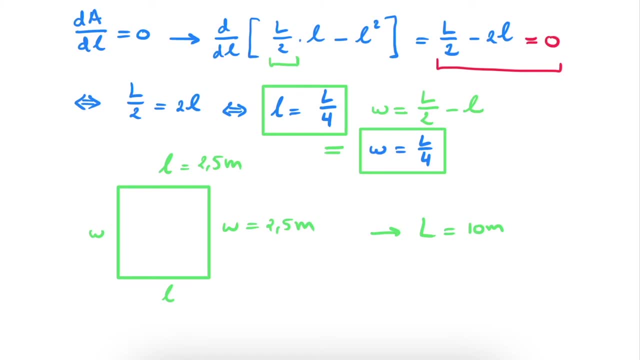 maximal surface enclosed is obtained by making a square surface and, just for good measure, the actual surface of the square- if your length has to be 10 meters is equal to the length of the square meters- is 6.25 meters squared, and we can even compare this if we had a rectangle with a length. 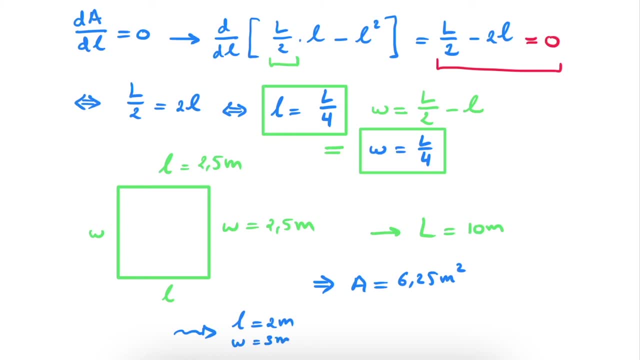 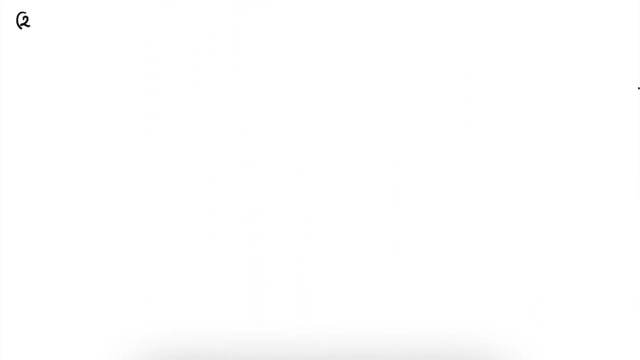 of two meters and a width of three meters, then we would have a surface equal to two meters multiplied by three meters, which is six meters squared, which is indeed smaller than the surface of the square. in the following exercise, we will look at a mathematical pendulum, and this is just a fancy. 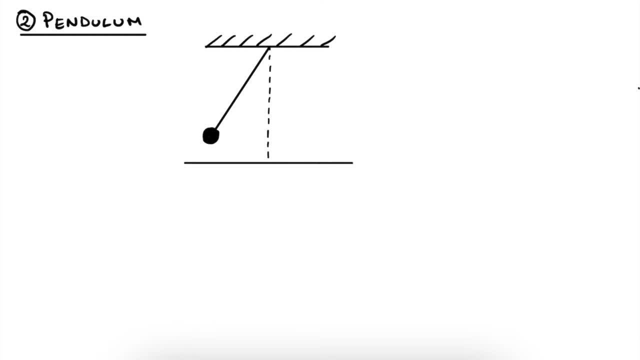 name for a pendulum that simply swings in one dimension, back and forward. and let me give you some more information about this pendulum. the length of this string is capital l, and the displacement of this pendulum compared to its resting position, where we just hang still, and 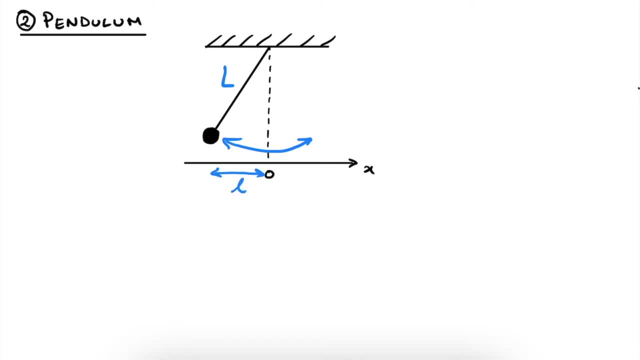 straight downward is called small l. now it turns out that the motion of this pendulum can be described very accurately. in normal words it would just be well back and forth. that's what a pendulum does, but in mathematics and physics it's described much more precisely by a mathematical equation. it turns out that it is very well described. 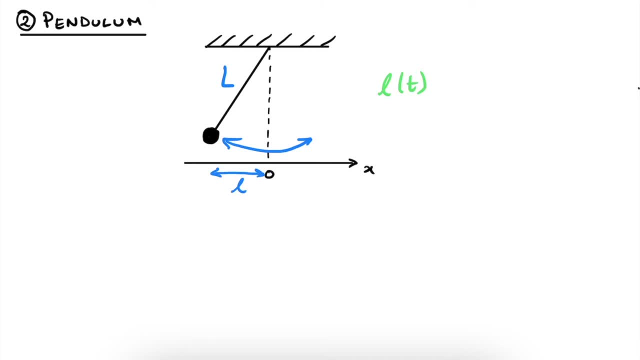 by describing the displacement of this pendulum through time, and this turns out- which i will leave for a future video on differential equations- that this is equal to alpha, which is just some constant which we could have easily put equal to one multiplied by the sine function of the following: the square root of g, which is the gravitational constant due to the 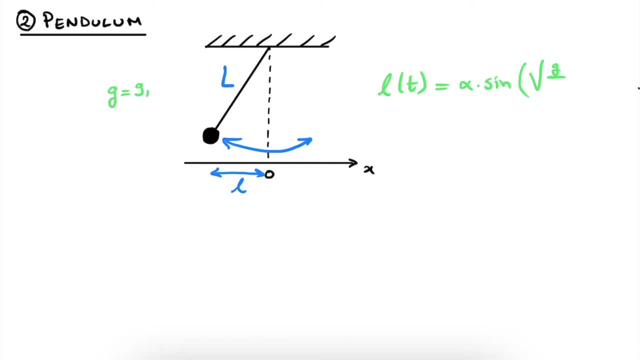 earth, and we know that g here on earth is 9.81 meters per second squared divided by the length of the pendulum, multiplied by the time. now this might look much more complicated than it actually is. let's look at it more deeply. this simply is a constant. it determines the frequency with which 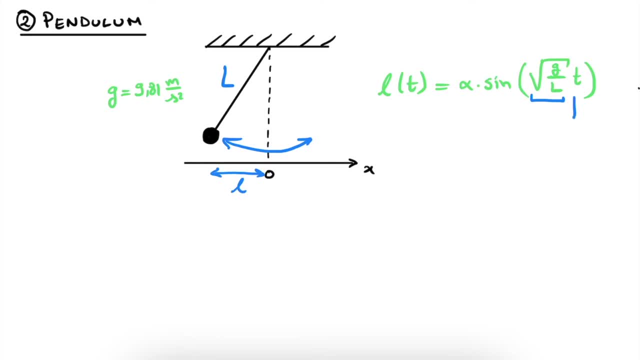 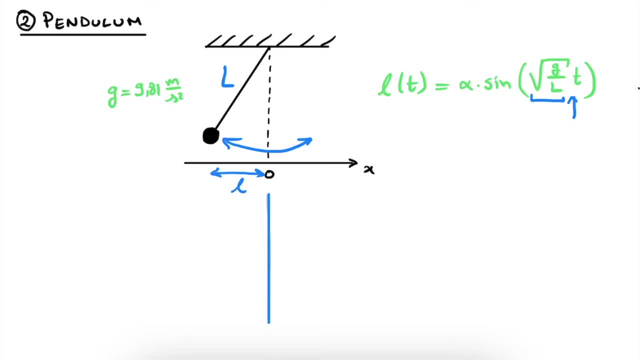 times t, and we know how the sign looks. if we, for example, plot the time in this direction, then we see that the pendulum, of course, when it starts right here, will simply oscillate like this in time, and this function we of course recognize as being the sine function and the frequency with which this pendulum oscillates back and forth. 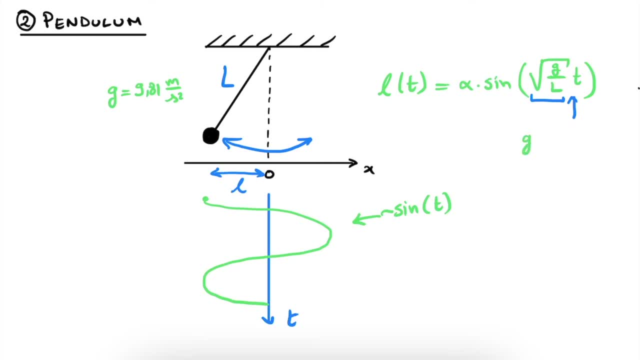 is determined by g, so the gravitational constant. so, for example, on the moon, a pendulum would swing much more slowly, and it's determined by the length of this pendulum. if the length is much larger, then the pendulum would also oscillate much more slowly. all right, so i described the motion of a pendulum. 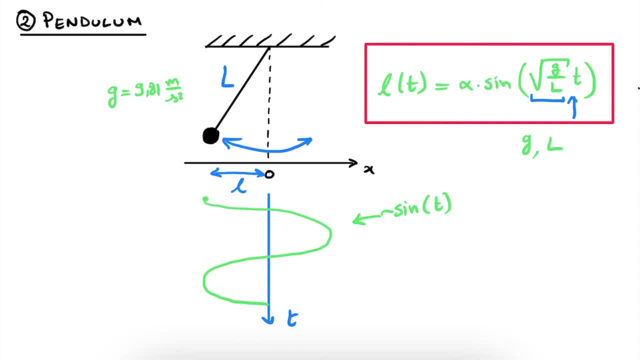 but there still hasn't been any problem yet to solve for us. i didn't ask you any question at this point. well, that's what i will do now. from this equation of motion, which describes the motion of the pendulum, can you find the time of one? 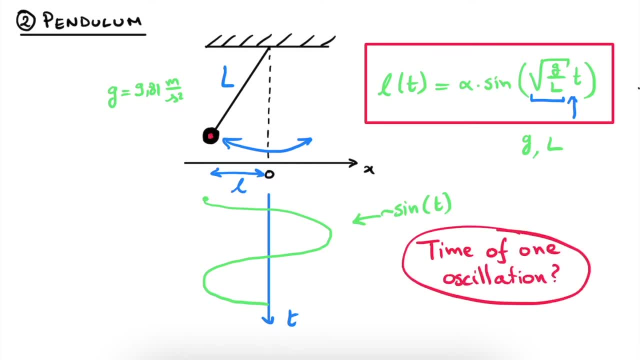 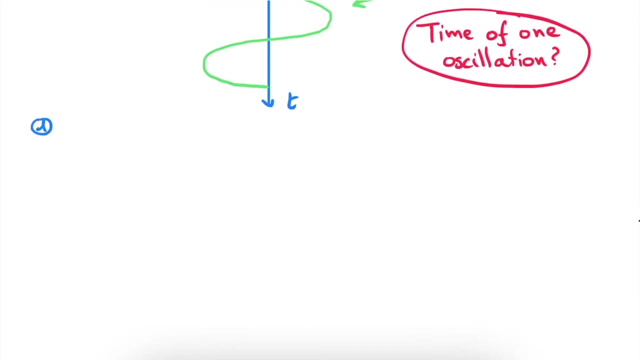 oscillation, meaning if i let loose of the pendulum right here, what is the time that it swings away and for it to come back again and this one turns out? we will be able to solve very easily with using derivatives, and let's see how that goes. first we identify how we can characterize the 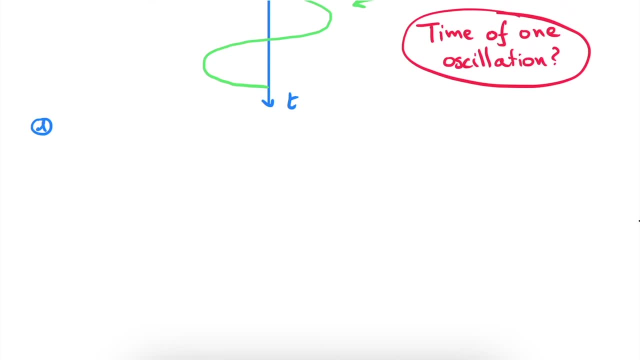 time of one oscillation? well, like i said, it would just be when the time of one oscillation? well, like i said, it would just be when i drop the pendulum and it swings away and then it comes back again. so what is characteristic of this motion? well, let's consider its velocity of the pendulum. we know that at its extremes, 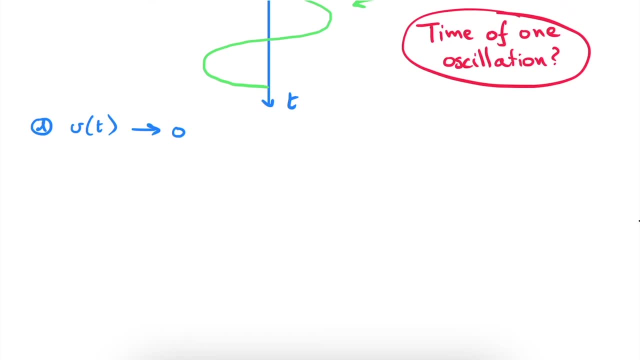 the velocity is equal to zero when it's at its maximum. therefore, what we need to find is the time between two extremes and then multiplied by two, because well, we're looking at one full oscillation and the time between two extremes is just going from one place. 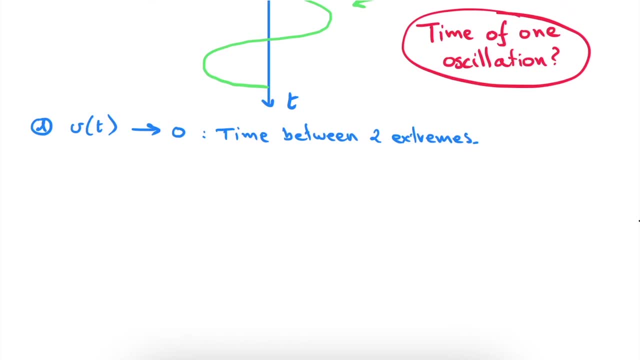 to the other, and to calculate the time between two extremes, we need to know, of course, at what time stamp these extremes occur. so at what time stamps the oscillator has a zero velocity, and it is at this point that derivatives come to rescue us, because we know that the 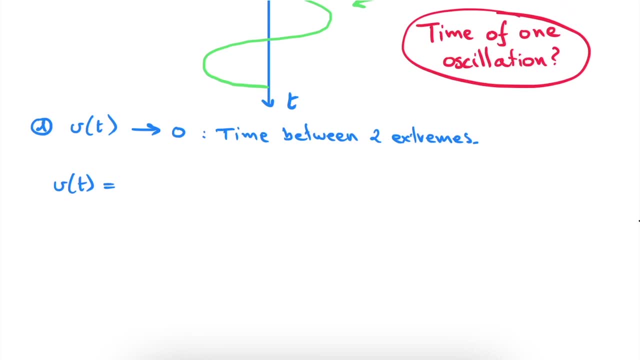 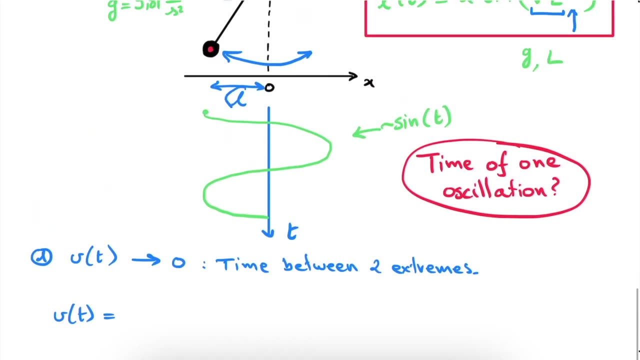 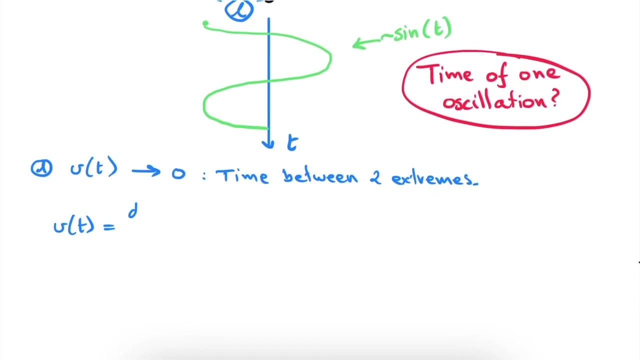 velocity of an object is equal to is the derivative of the position of this object to the time, and in this case the position of our object is simply this displacement term. so we know that the derivative, or the velocity of our pendulum is equal to the derivative to time of the following: l of t, the displacement in time of our pendulum. and since 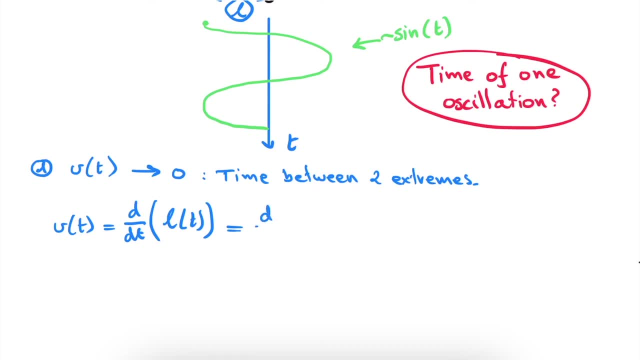 we know the expression of the displacement of our pendulum, we get the following derivative that we need to solve: we have, of course, this alpha, which was a constant multiplied by the sine of again another constant, g divided by capital, l multiplied by t- the time, and we see here that the only variable to which we are deriving occurs. 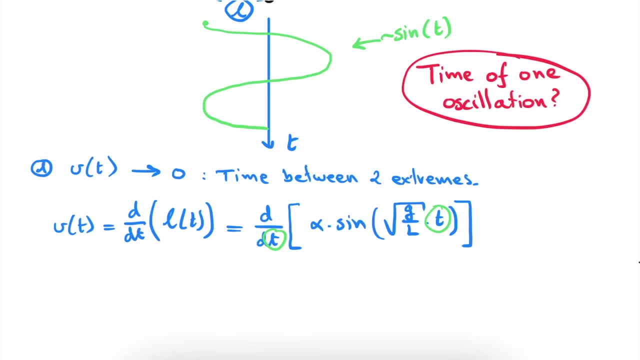 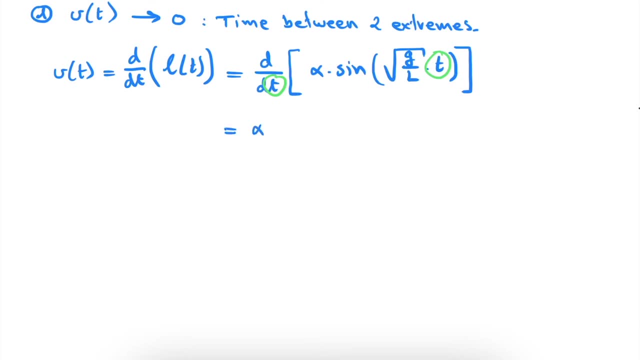 here in this sine function. and now we can very easily take this derivative using the derivative of a sine function and the chain rule. we have of course this alpha, which is a constant and can be put outside of the derivation. then we multiply this with the derivative of this sine function. 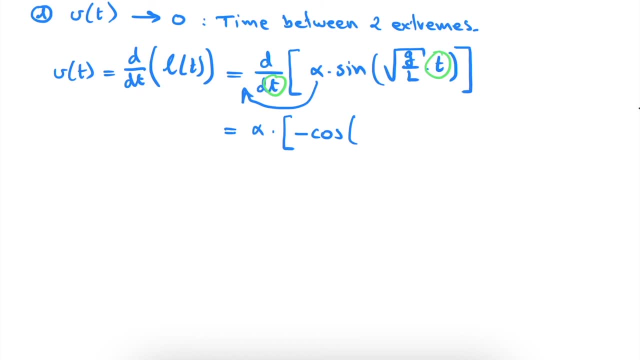 which is minus the cosine function of the same angle, in this case the square root of g divided by l multiplied by t. however, we're not done yet here, because we have to use the chain rule, because this t is still glued to this factor in front of it, which is the square root of g over l, which is just a constant. 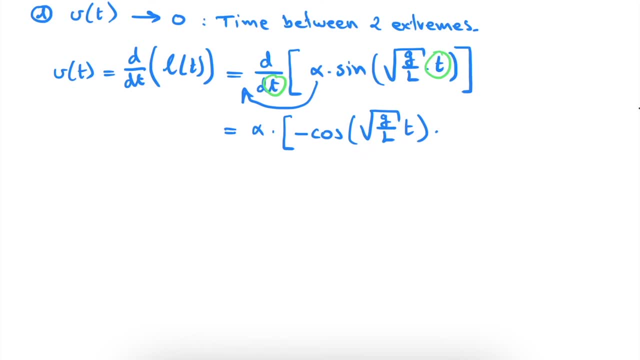 so deriving this entire thing to t will simply give us this constant again, which is g divided over capital l, and taking the square root of g over l and taking the square root of g over l, we can see that we now have an expression for our velocity. our velocity changes in time according 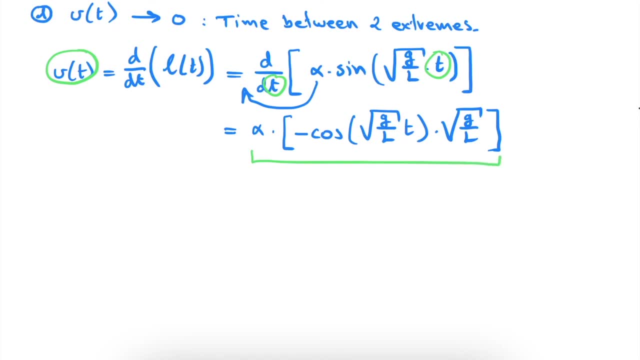 to this function. and again this function looks much more difficult or complex than it actually is. let's rewrite it to get a more clear picture. so we have minus alpha multiplied with this other constant, g, divided by capital l, and now we multiply this simply with a cosine of again this constant. 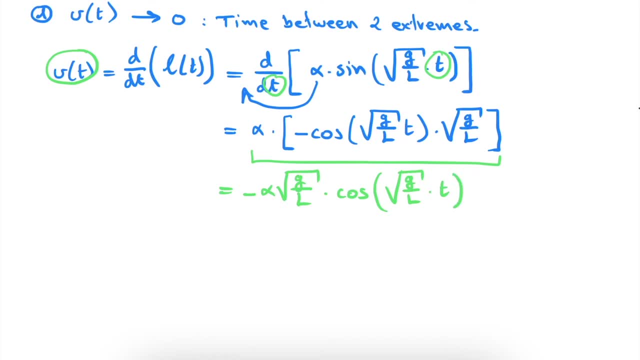 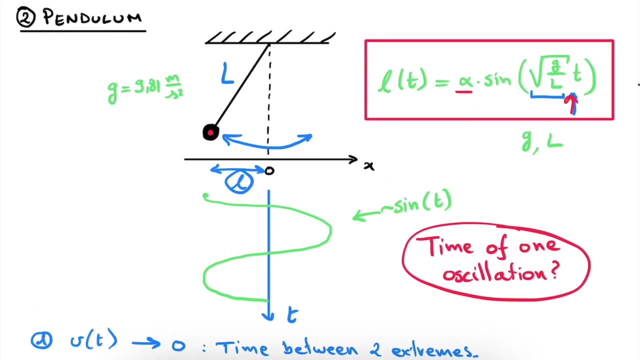 g divided by capital, L multiplied with t. And we see that the only difficult or only changing part in this solution is this variable, t. So where the displacement was a sine function of time, right here we see that the displacement also had this constant in front of it. 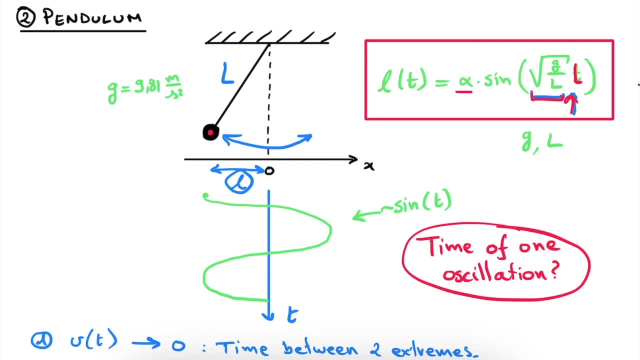 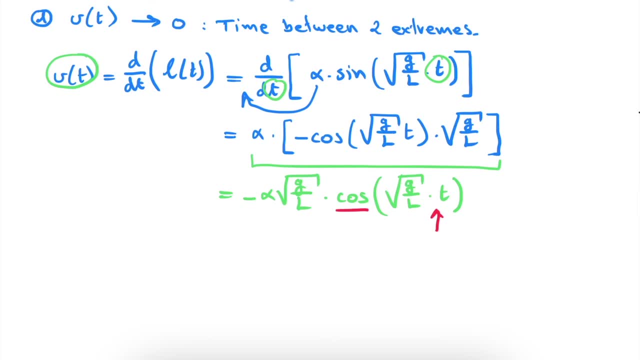 this constant inside of the sine, but ultimately only changes when this t changes. We see that the velocity of our oscillator changes with the cosine of this same t, And now that we have an expression for our velocity, we can of course also see: 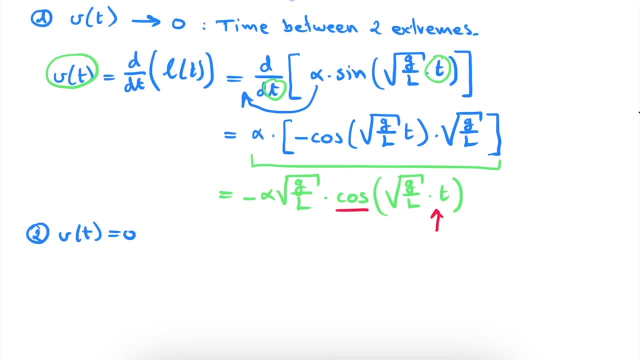 where our velocity is equal to zero. For this we need, of course, to determine where the cosine is zero. Well, we know very easily where a cosine is zero. The cosine of any angle is zero for the following cases: We have pi over two, we have three pi over two, and so on. 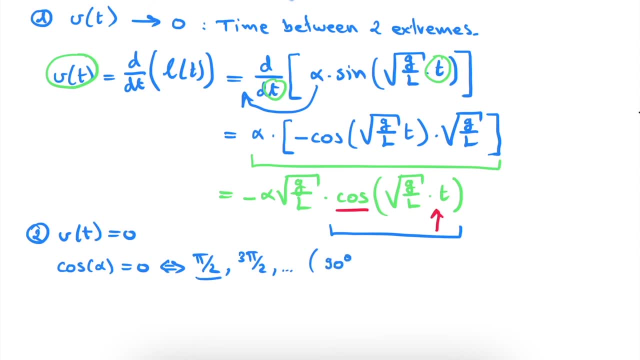 And this basically means 90 degrees, which is pi over two. We have 270 degrees, which is three pi over two, plus any number times 180 degrees, of course. So when alpha is equal to all of these cases, then our cosine will be zero. 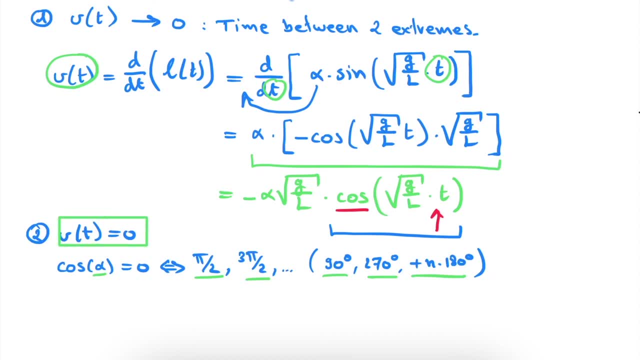 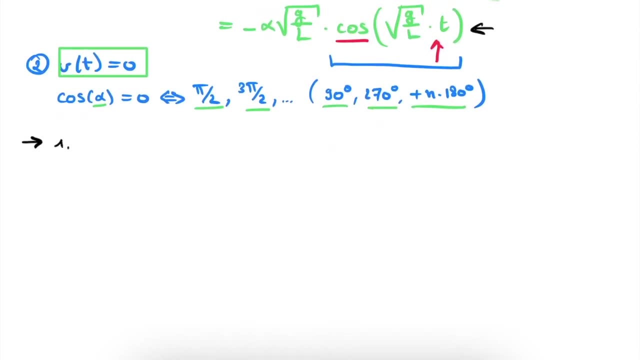 and therefore our velocity will be zero. So let's see what this concretely becomes for our solution right here. So the first time that this cosine is equal to zero is when t is equal to the square root of L divided by G multiplied by pi over two. 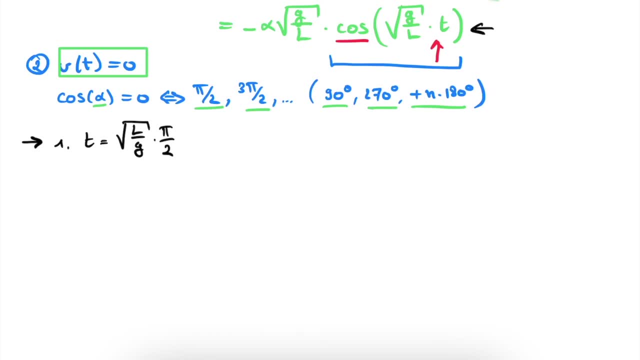 And now you might wonder: well, why is this exactly true? Well, if we simply fill in this t in the argument of our cosine, then we get the following: We have the cosine of well, simply writing the square root of G divided by capital, L multiplied with t. 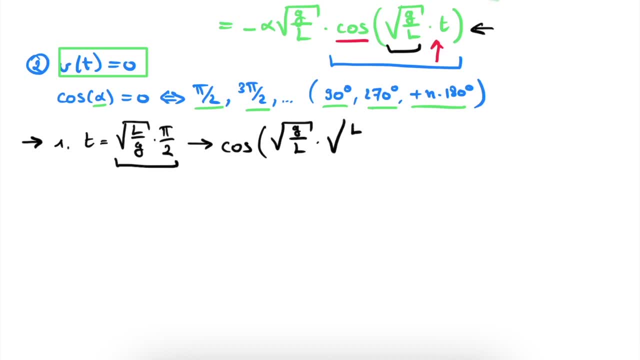 t is simply equal to this right here. So we copy this capital: L divided by G, multiplied by pi over two. We see that this term and this term multiply with each other to simply become one, which leaves us with the cosine of pi over two. 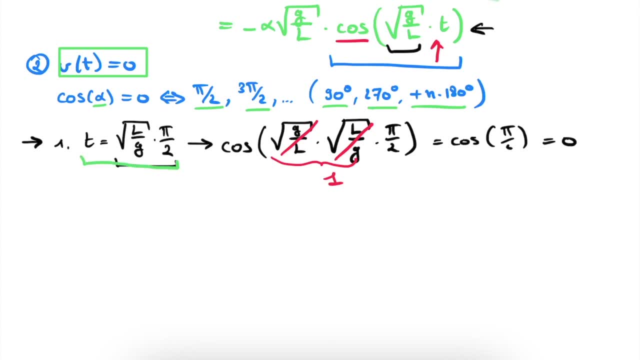 which is simply zero, And therefore for t is equal to this number right here, the cosine will be zero and therefore the velocity will be zero. So that's already a first solution. For the second solution we have, t is equal to. 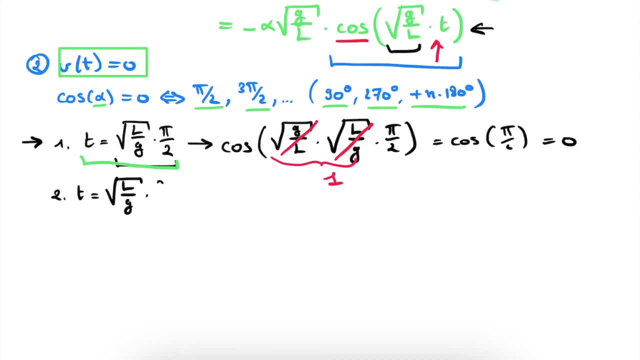 the capital L divided by G, multiplied by three, pi over two, which is now simply this solution right here. Because, again, if we fill this in in the same fashion as before, we get indeed zero, And of course we see a pattern here that at each time step. 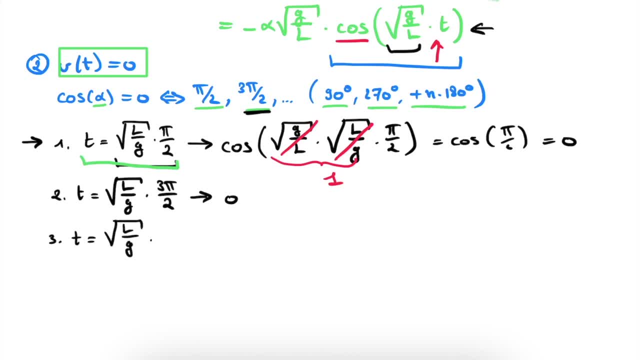 where t is equal to capital L divided by G, multiplied with an odd multiple of pi divided by two, we get that our velocity is zero And if we draw this out on our sketch, what this actually means, because it's always important to keep an intuitive feeling of what we're doing here- 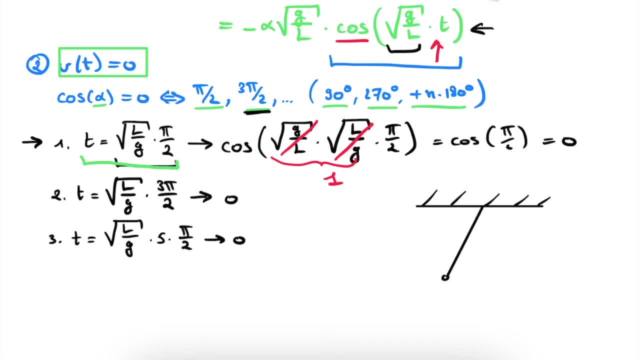 then we see that in the first case where our velocity is zero is simply at the start, when our pendulum is not moving because, well, we're holding it quite still, And then if we let go of the pendulum, we see that it will swing all the way. 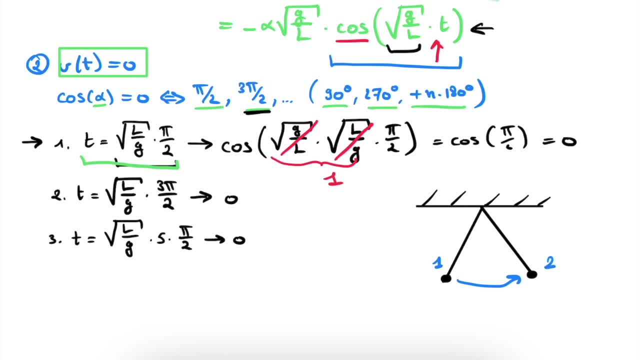 to the other side before it comes to a halt again- And this number two corresponds to this time step where the velocity is again zero. then again accelerating from a halt and swinging back again, we will have this third situation, which is this one where the velocity is also zero, and it will 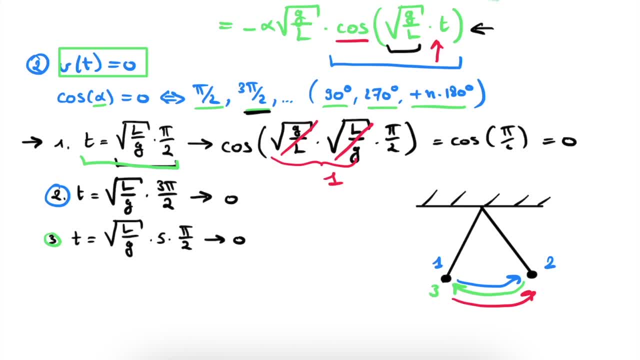 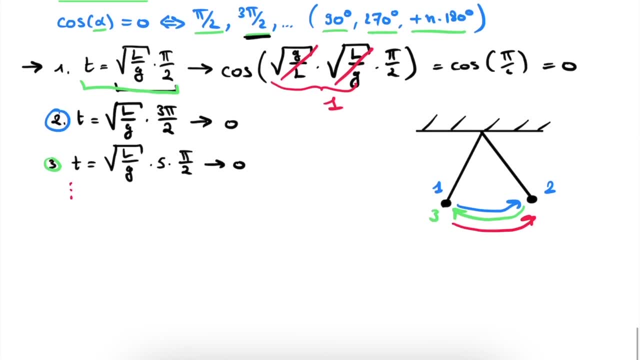 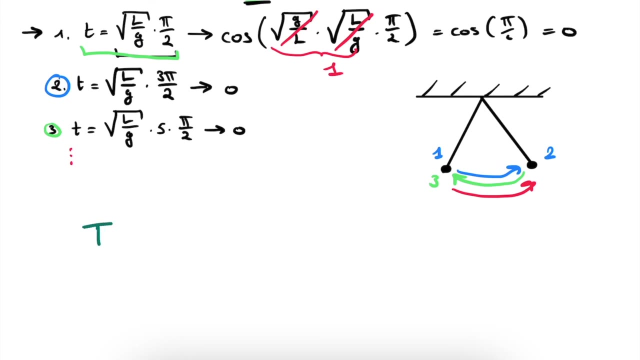 go on endlessly going back and forth, and each time a maximum is reached, the velocity will be zero. so how do we now calculate from this the time between two maximums or the time for an entire oscillation? well, from what we found, we see that the entire time for one oscillation is simply three minus one. 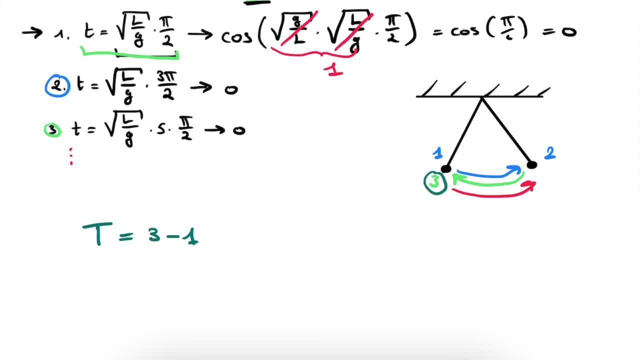 with which i mean is the timestamp for this situation minus the timestamp for this situation, and we have the timestamps for those two situations. it's simply this timestamp minus this timestamp, because at that point our oscillator has swung away and back again. so if we fill this in, we have the square root of l divided. 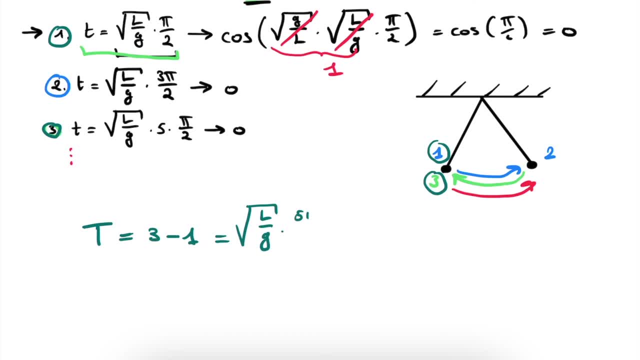 by by g multiplied by 5 pi over 2, minus the square root of L divided by g multiplied with pi over 2.. This can be rewritten as the square root of L divided by g multiplied by 5 pi over 2, minus pi over 2, which in the end is equal to 2 pi multiplied with the square root of L divided.